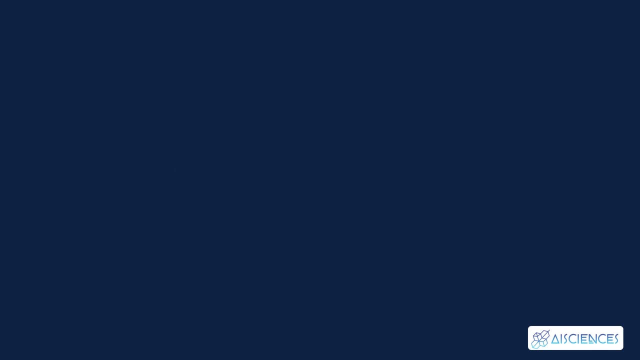 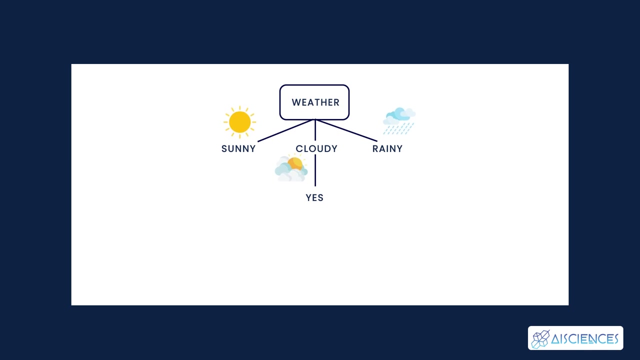 is, then it goes to the next node attached to that decision In the diagram. the tree will first ask what is the weather? Is it sunny, cloudy or rainy? If yes, then it will go to the next feature, which is humidity and wind. It will again check if there is a strong wind or weak. if it's a weak wind and 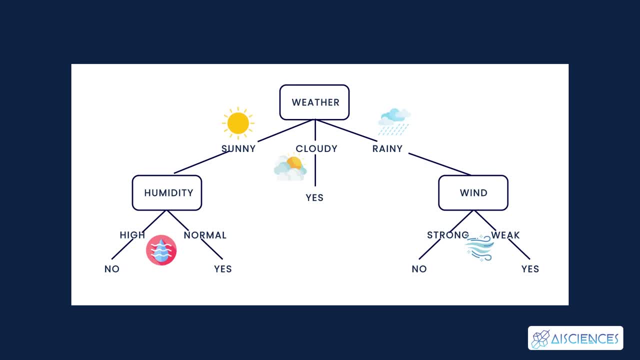 it's rainy, then the person may go and play. Did you notice anything in the flowchart? We see that if the weather is cloudy then we must go to play. Why didn't it split more? Why did it stop there? To answer this question, we need to know about a few more concepts like entropy. 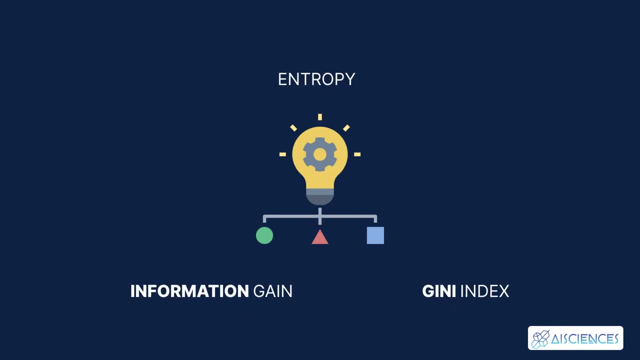 information gain and Gini index. But in simple terms, I can say here that the output for the training dataset is always yes for cloudy weather. since there is no disorderliness here, we don't need to split the node further. The goal of machine learning is to decrease uncertainty. 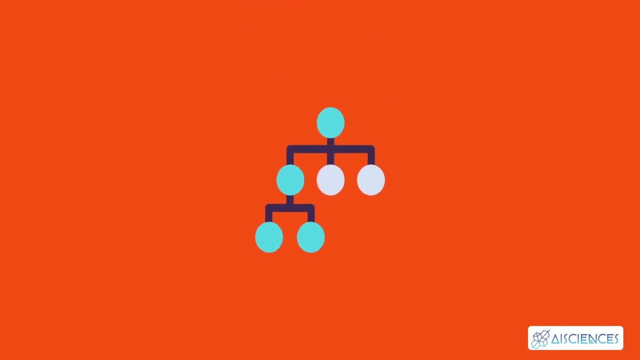 or disorders from the dataset, and for this we use decision trees. Now you must be thinking: how do I know what should be the root node, What should be the decision node? When should I stop splitting? To decide this, there is a metric called entropy, which is the 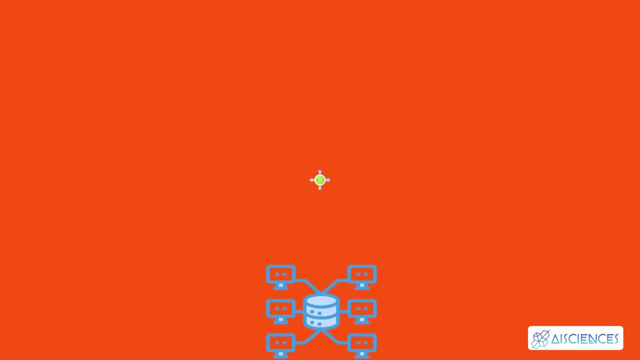 amount of uncertainty in the dataset. Entropy is nothing but the uncertainty in our dataset or measure of disorder. Let me try to explain this with the help of an example. Suppose you have a group of friends who decides which movie they can watch together on Sunday. There are two. 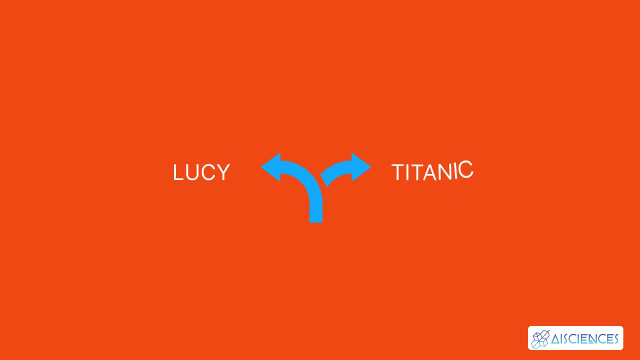 choices for movies. one is Lucy and the second is Titanic, and now everyone has to tell their choice. After everyone gives their answer, we see that Lucy gets four votes and Titanic gets five votes. Which movie do we watch now? Isn't it hard to choose one movie now? 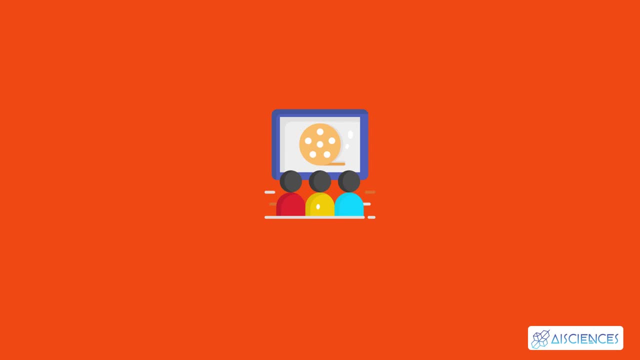 because the votes for both the movies are somewhat equal. This is exactly what we call disorderliness. there is an equal number of votes for both the movies and we can't really decide which movie we should watch. It would have been much easier if the votes for Lucy were eight. 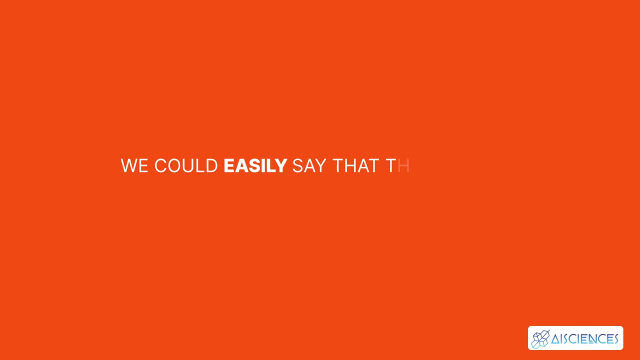 and for Titanic, it was two. Here, we could easily say that the majority of votes are for Lucy. hence, everyone will be watching this movie. Now we know how decision tree works, but Titanic is the only movie that can be watched. Now we know how decision tree works, but Titanic.